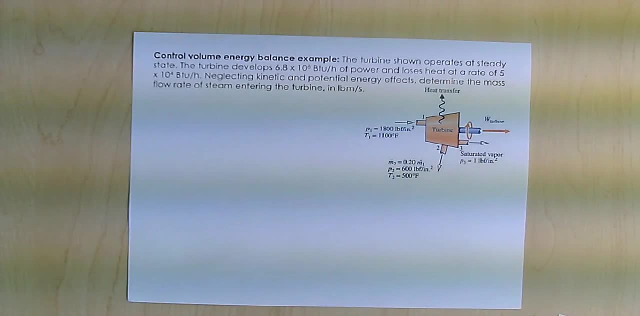 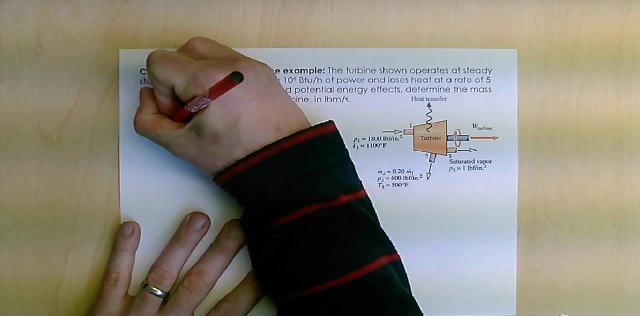 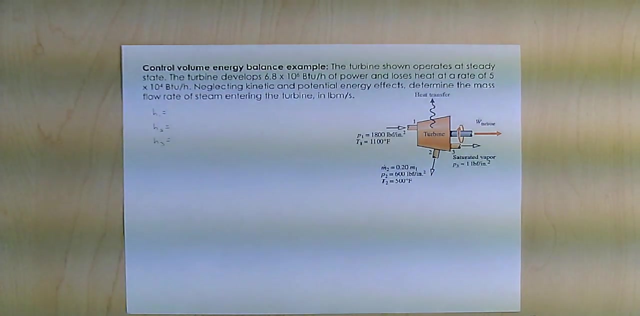 So the first thing I need to do in this problem is I need to calculate my H values. So I'm going to go look up, I'm going to go look up H1,, H2, and H3 from my systems here and I've got basically two properties, so I should be able to find any other one, okay. 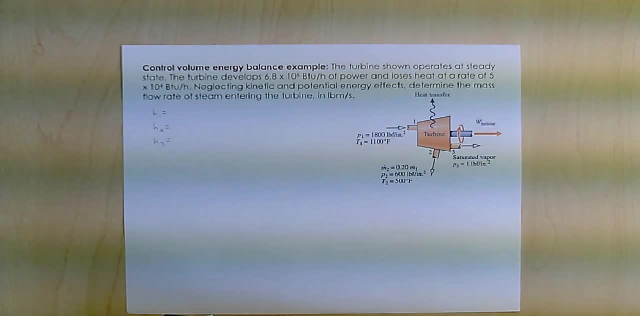 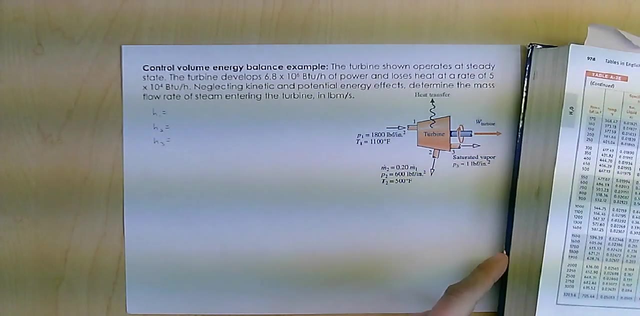 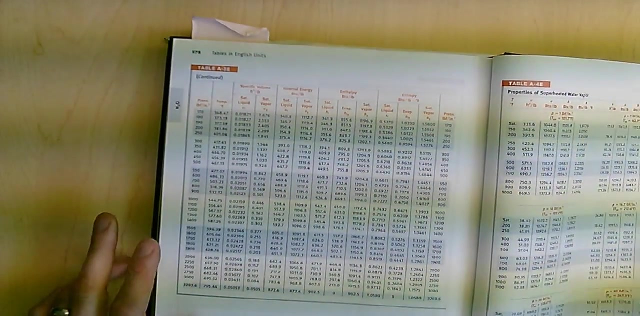 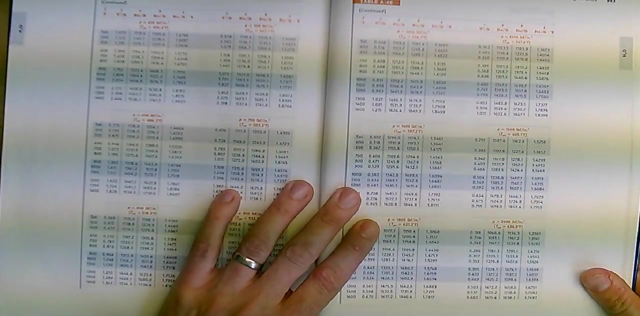 So I'm going to start. This is water Steam. yep, This is water at 1,800 PSI and 1,100 Fahrenheit. So at 1,800 PSI- oops, We will be over here, Go to 1,800.. So in this table- this is table A4E- 1,800 and 1,100, okay. 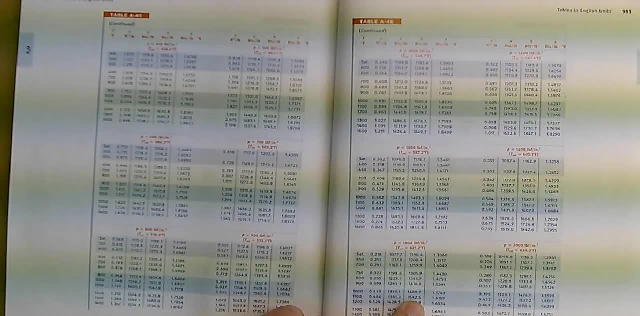 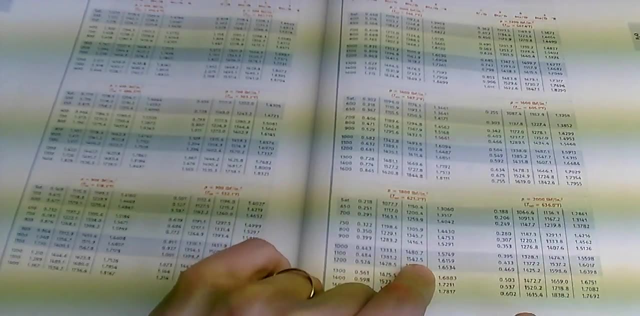 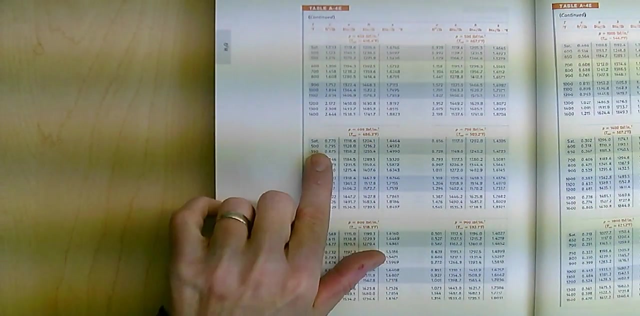 My H value is 1,542.5,. okay, State 2,, I have a pressure of 600 and a temperature of 500, so I'll go to 600 right here, And my H value is 1,216.2.. 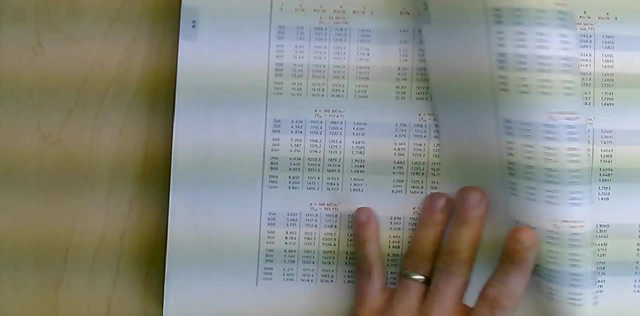 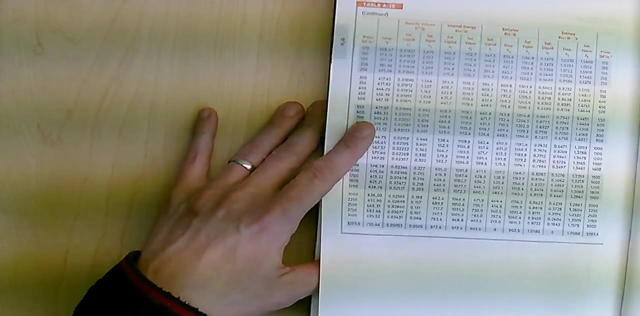 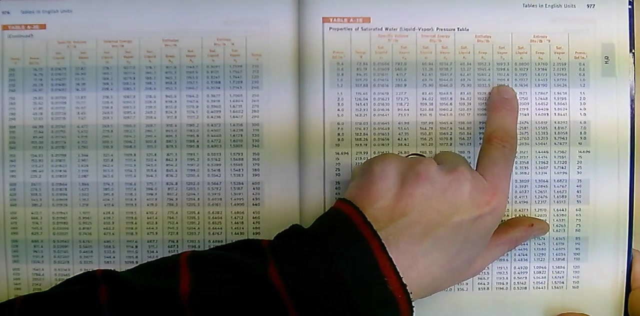 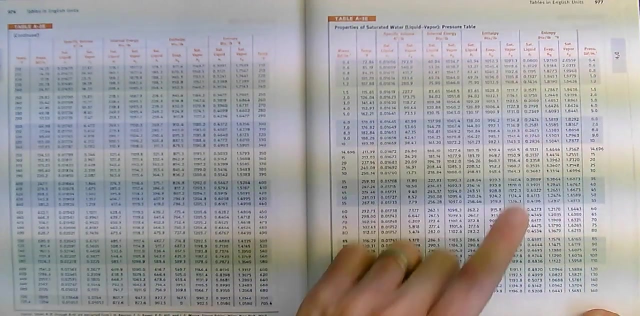 State 3 is saturated vapor at 1 PSI. So I come over here to state, I come to my pressure table. 1 PSI saturated vapor enthalpy is 1,105.8.. So I have all of those. I've set my states. I've found the enthalpy for each state. 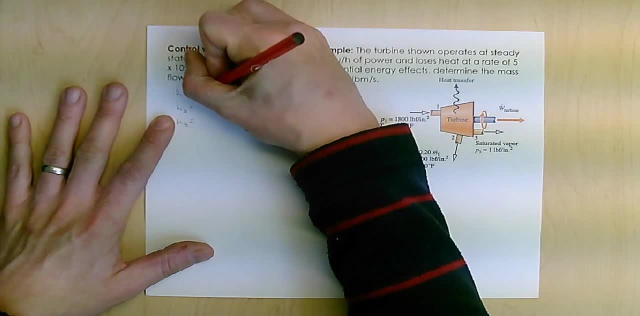 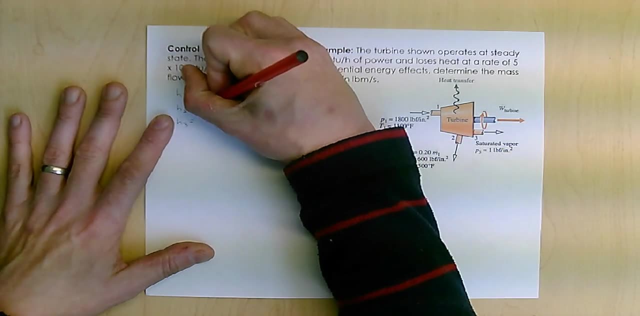 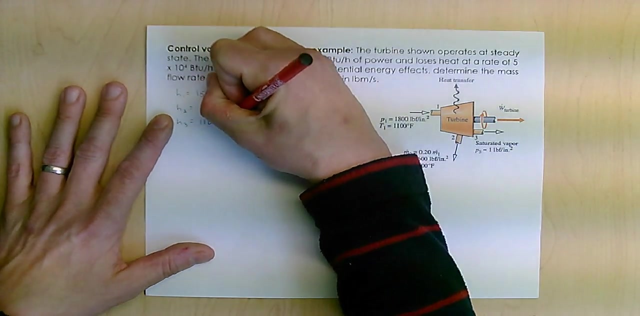 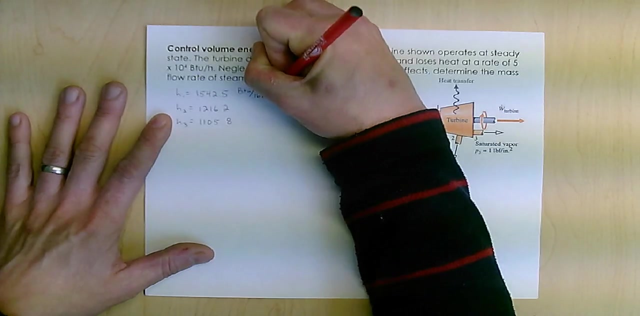 So again, this was 1,542.5.. H2 was 1,216.2.. State 3 was 1,105.8, and these are all BTUs per pound. Okay, So that's the first step of the problem. 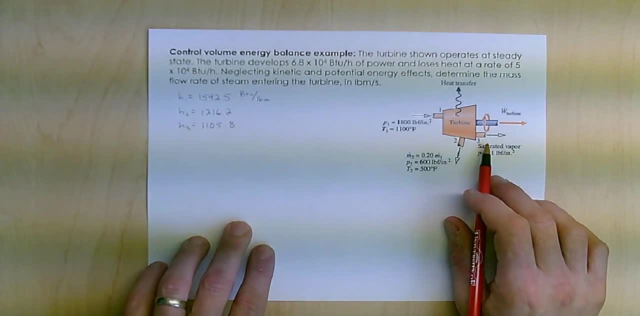 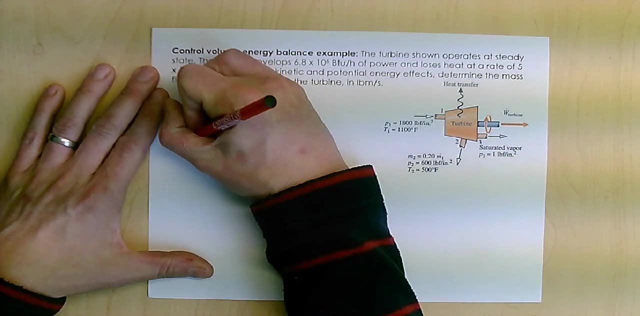 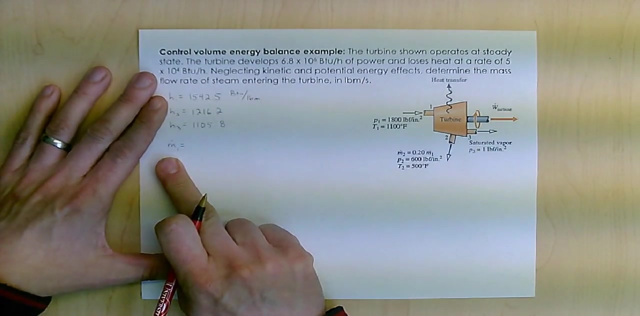 So now I know all of my H values for each of the states. The next thing I need to do is develop this conservation of mass principle, which basically states that the inlet mass equals the outlet mass for steady state. So that means M.1 equals M.2 plus M.3, right? 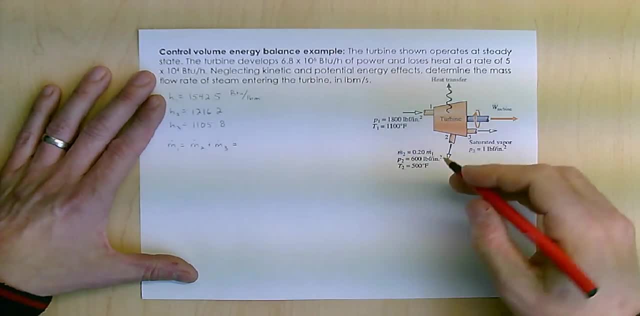 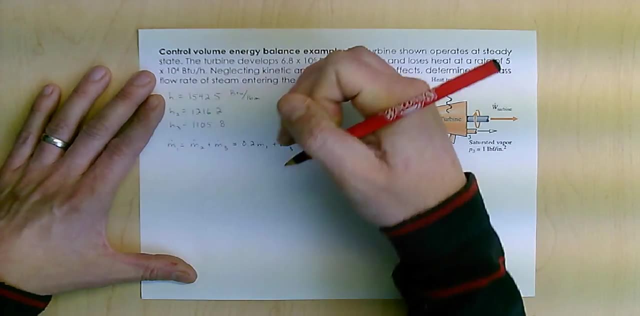 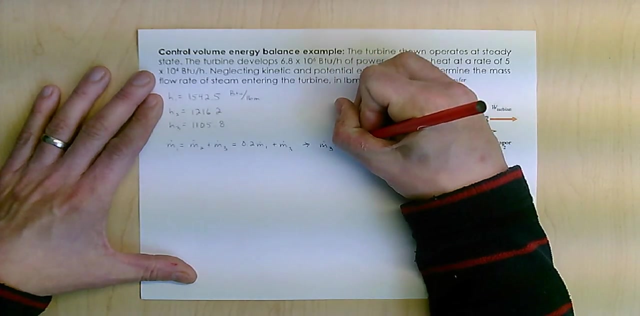 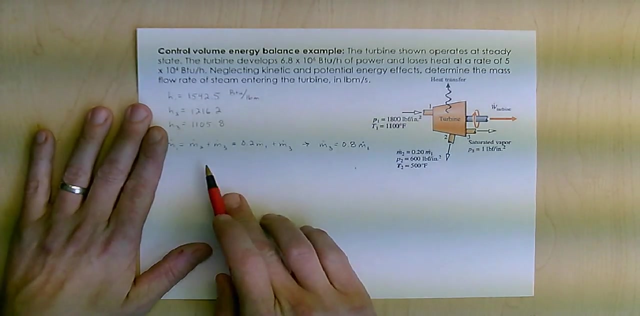 Okay, M.2 is 0.2 M.1 plus M.3.. From that I learn that M.3 has to equal 0.8 times M.1.. So I don't know the mass flow, but I've got them all related to the incoming mass flow, right. 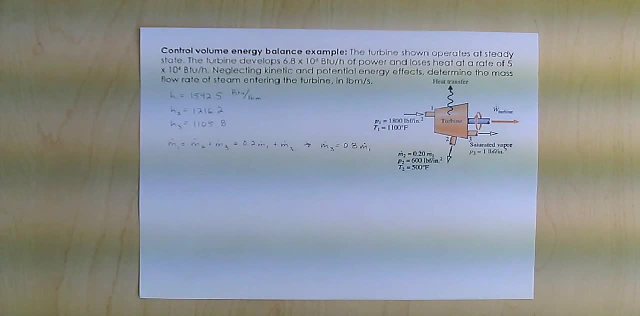 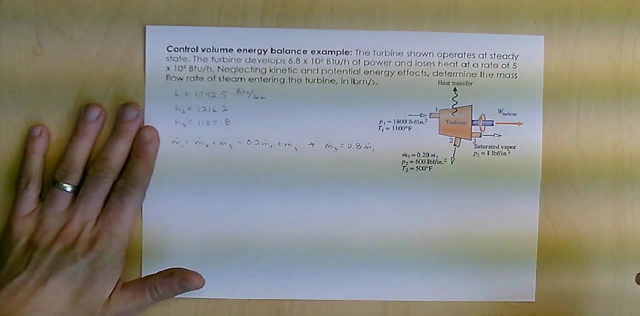 20% goes this way, 80% of it goes that way. That's essentially what we've got here And again, that's because the mass flow in has to equal the mass flow out. Okay, So now we move to our first law equation, right? For steady state, the change in energy is 0. I have no potential or kinetic energy effects, So all I really have is Q dot minus W dot plus mass flow in H in minus mass flow. So out exit times, H exit right. 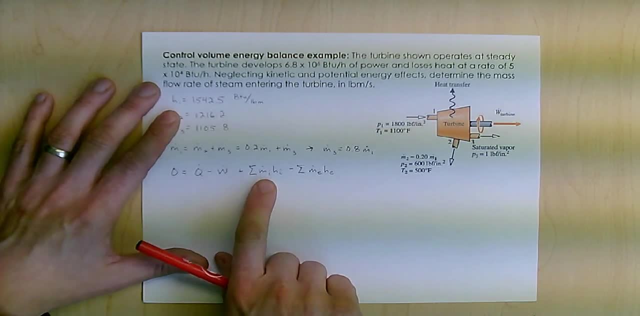 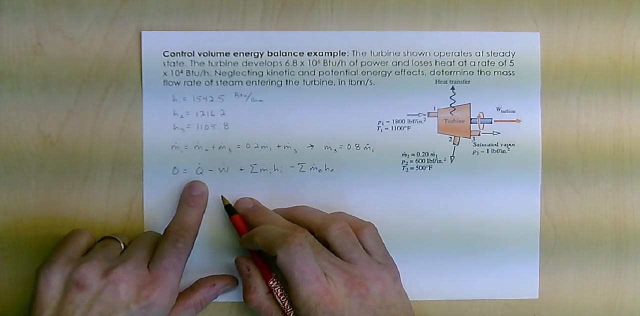 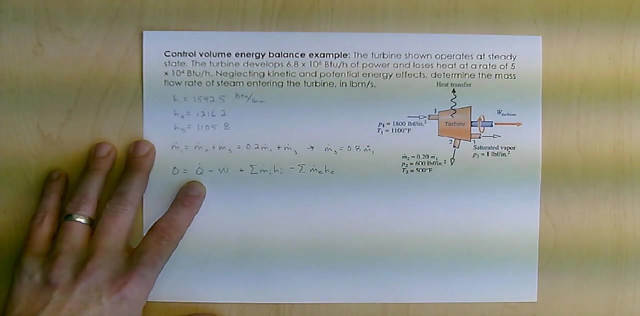 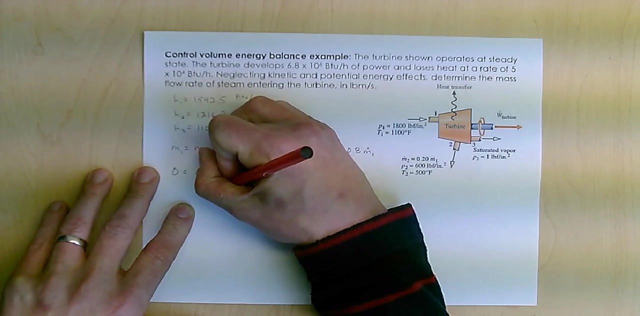 So again, it's heat minus work plus, basically the enthalpy in minus the enthalpy out, And I know everything in this equation, which is to say Q is 5 times 10 to the 4th, That would be BTUs per hour. 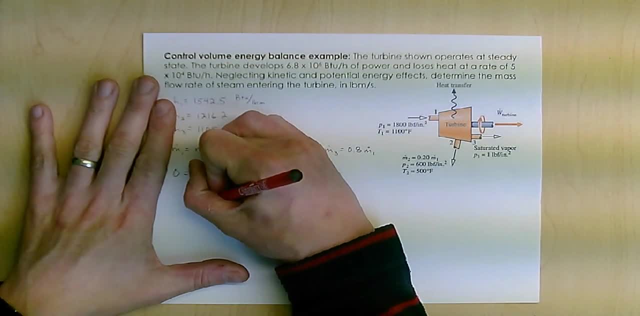 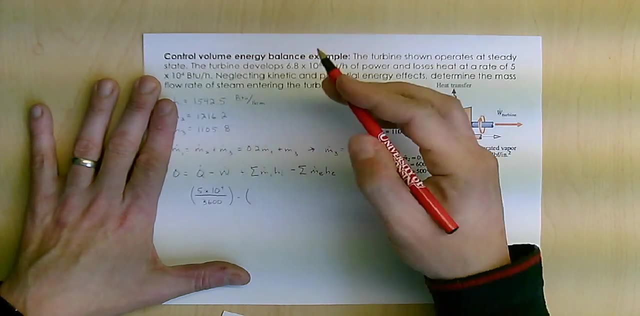 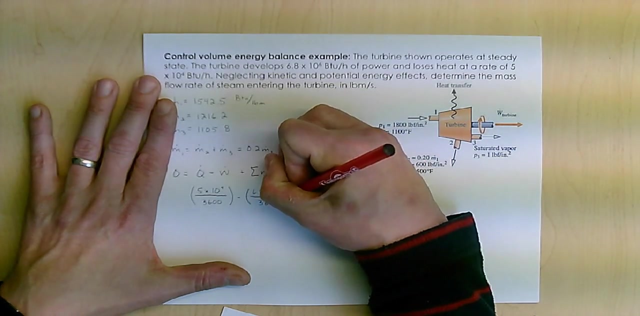 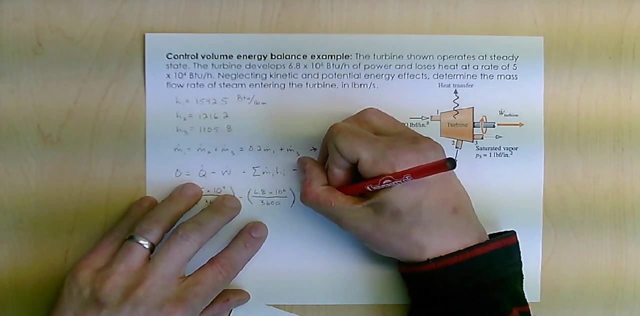 So I divide that by 3600 to get everything in seconds. So that's Q minus the work, which is going to be 6.8 times 10 to the 6th divided by 3600.. Plus the mass flow in which is. 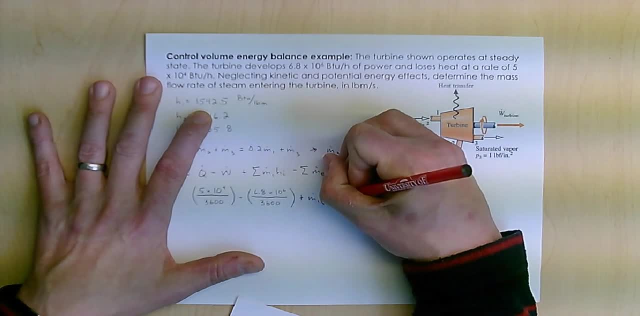 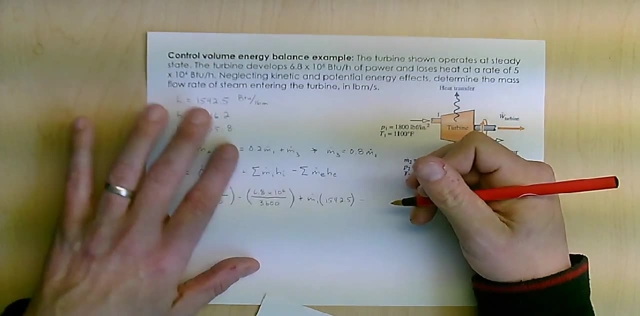 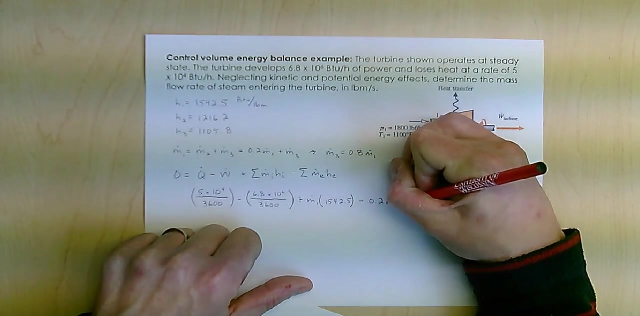 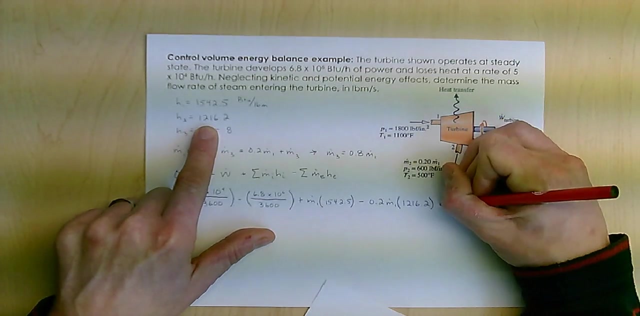 M1 times H1, which is 1542.5 minus the mass flow out, which is: I've got two of them, I've got 0.2 mass flow 1.. That is for H2, so that would be 1216.2 minus 0.8 mass flow 1 times. 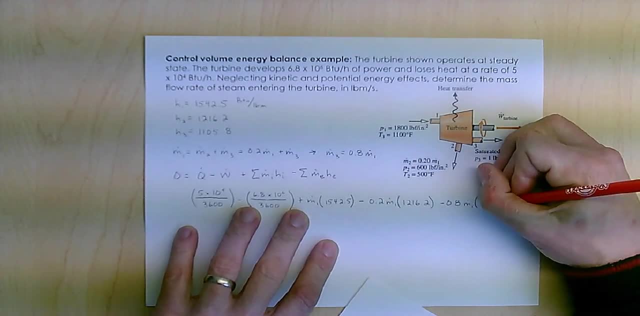 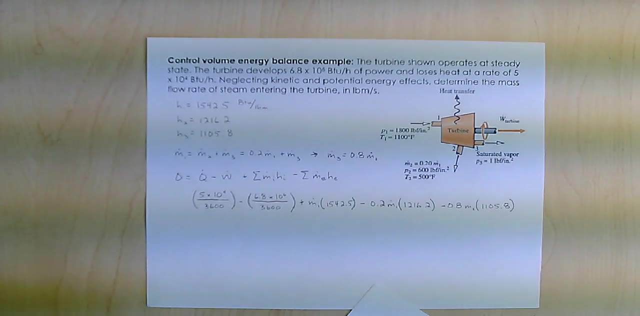 Again, that's How much is flowing out at state 3, which is 1105.8.. So I've got a big equation. Everything's in BTUs, pounds and seconds, right. So Q minus W. enthalpy in minus enthalpy out.